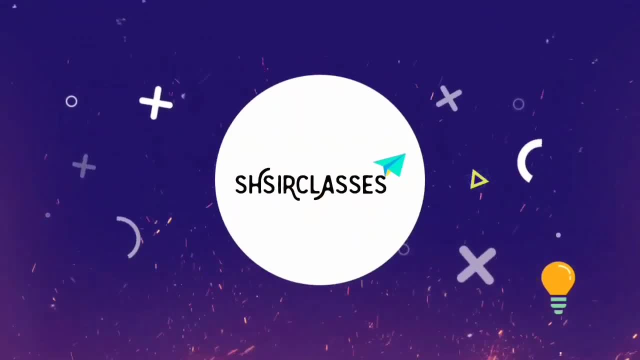 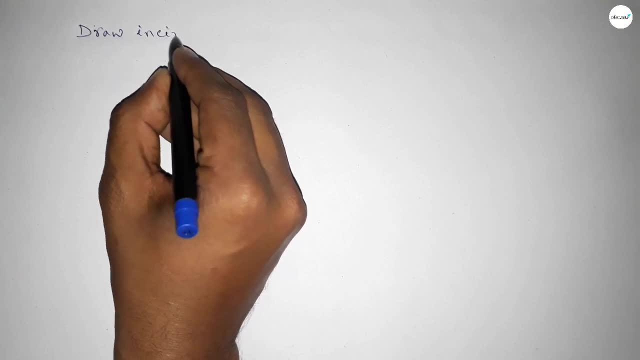 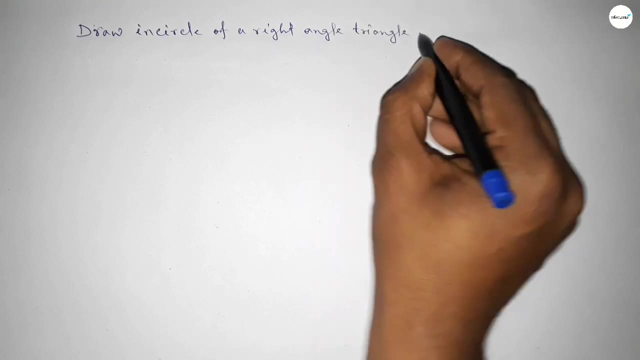 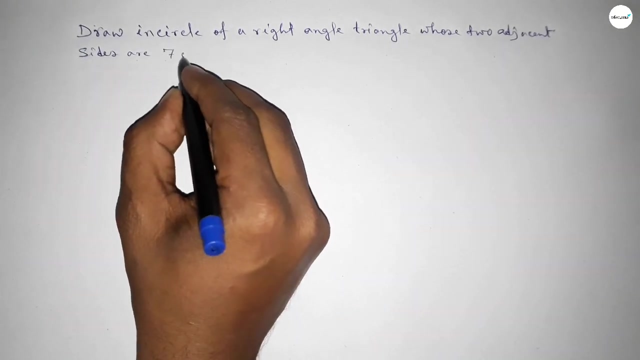 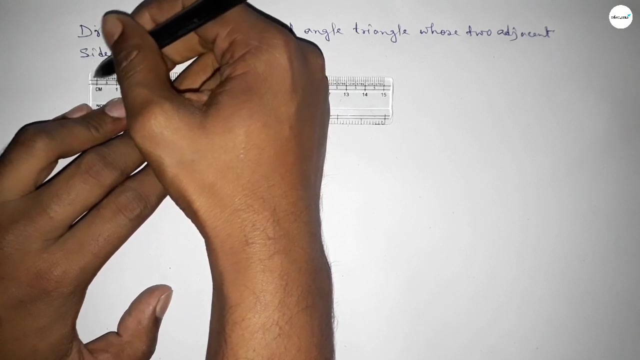 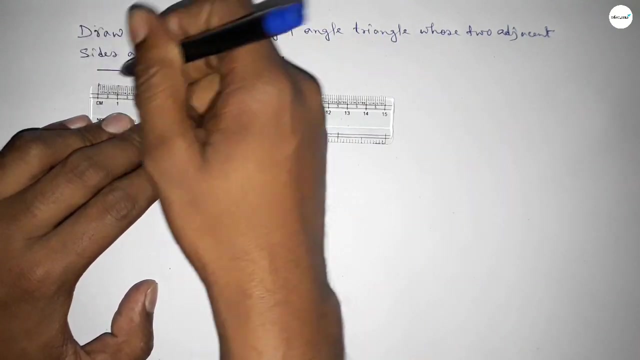 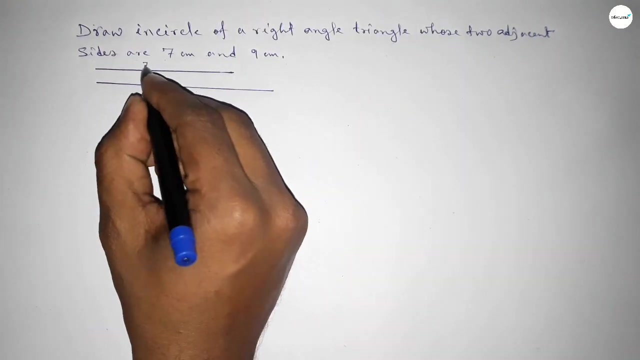 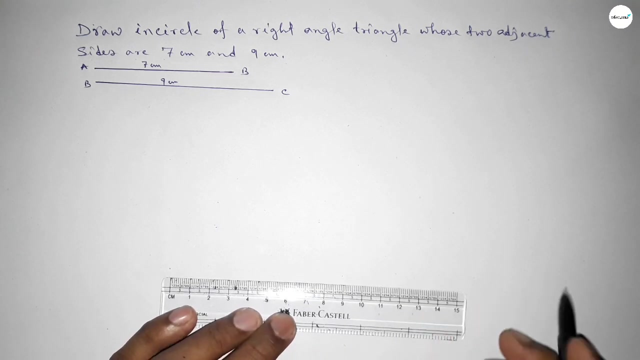 Hi everyone, Welcome to EssayShare classes Today. in this video we have to draw in circle of a right angle triangle whose two adjacent side is 7 centimeter and 9 centimeter. So let's start the video. So first of all, drawing here the length, 7 centimeter, So this is 7.. So first drawing 7 centimeter line, Then drawing 9 centimeter line, So this is 9 centimeter, Okay, and this is 7 centimeter and this is 9 centimeter. And taking this AB line and this is BC line, Okay, 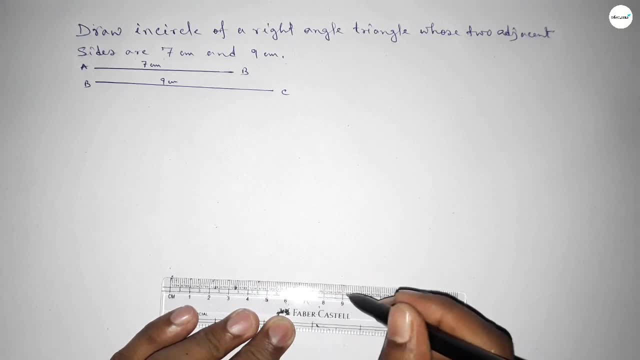 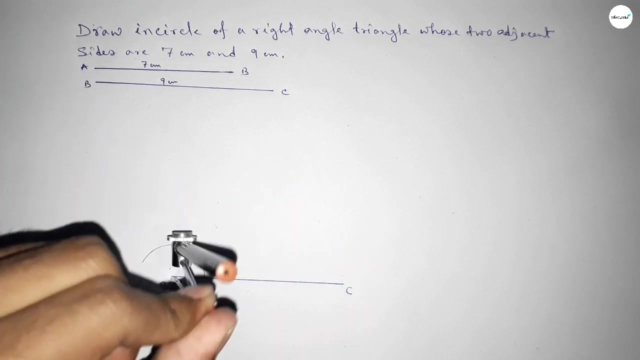 Now first, drawing here, 9 centimeter length First, so this is 9.. drawing here the line bc, 9 centimeter, so this is b c line. next we have to draw a 90 degree angle on the point b, so taking any length, and drawing an arc by this way, with same length, and putting. 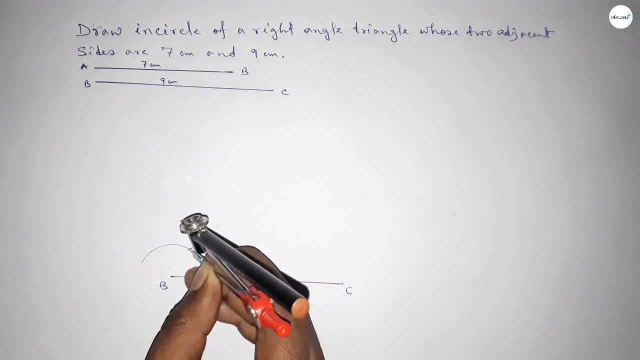 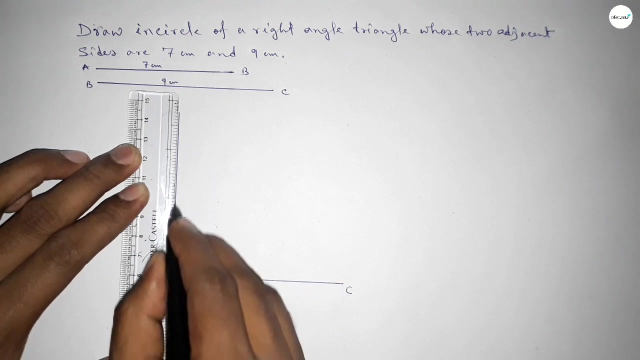 the compass here and cut here with same length. and putting the compass here and cut here. and drawing arc here with same length and putting the compass here and cut here so both the curve intersect at a point, now joining this to get here a 90 degree angle. so we got a 90 degree. 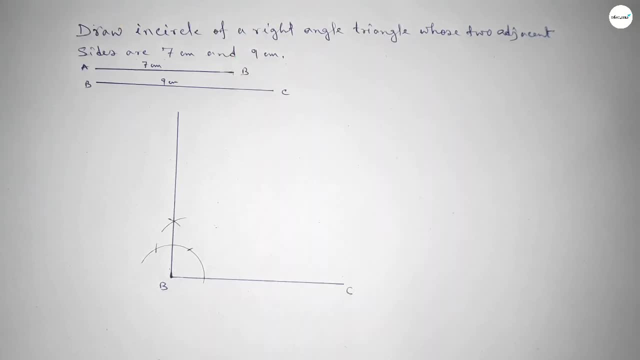 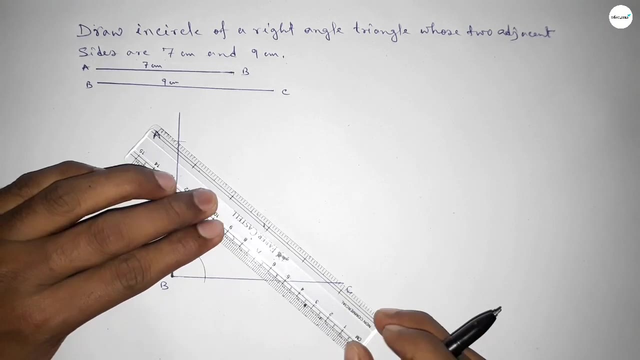 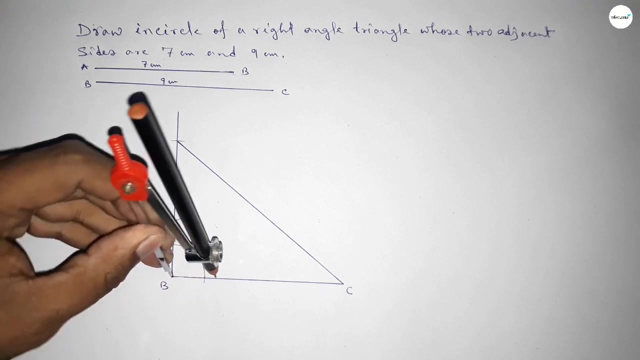 now taking the length ab 7 centimeter, so putting the compass here and cut here. so here, taking a point, now we have to join ac. so we got a right angle triangle. okay, now we have to bisect the angle b. so taking the bc- 9 centimeter, and drawing an arc here with same length and putting the compass here with same. 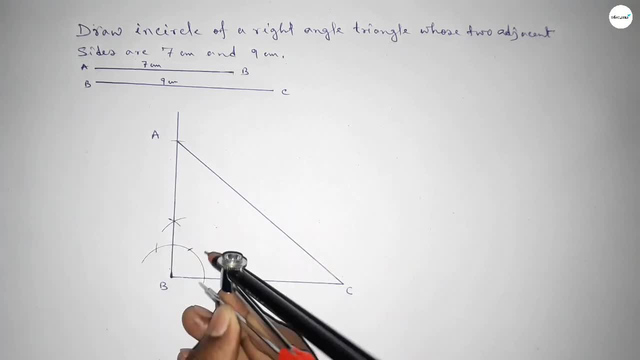 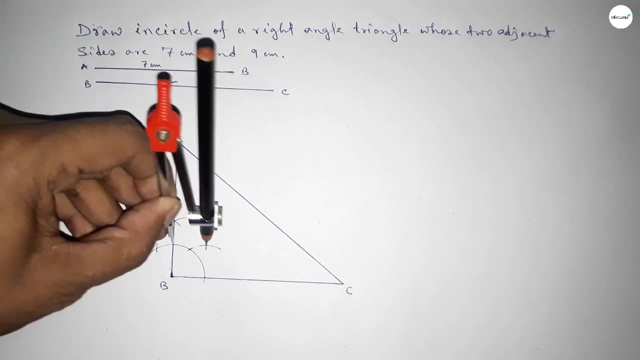 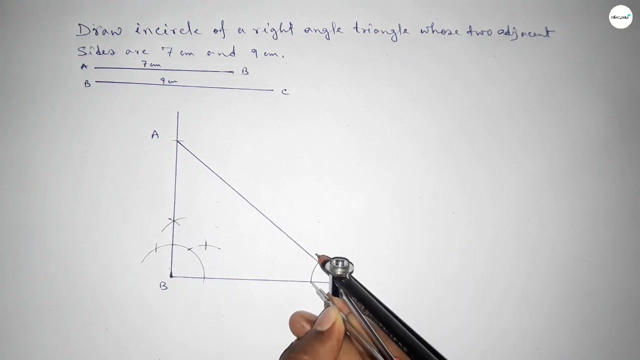 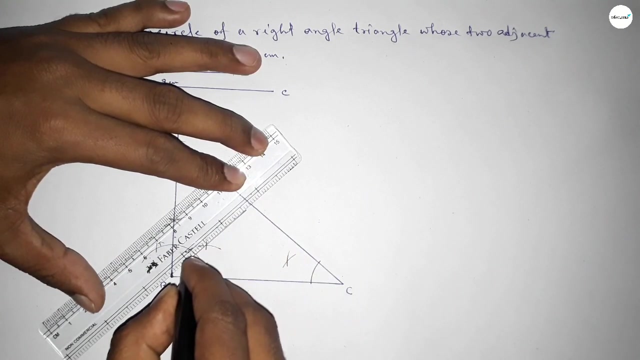 length and putting the compass here and cut here and drawing an arc here with same length and putting the compass here and cut here again with same length. you can take any radius to draw arc here, okay, with same length, and putting the compressor and cut here. now joining this bisector.